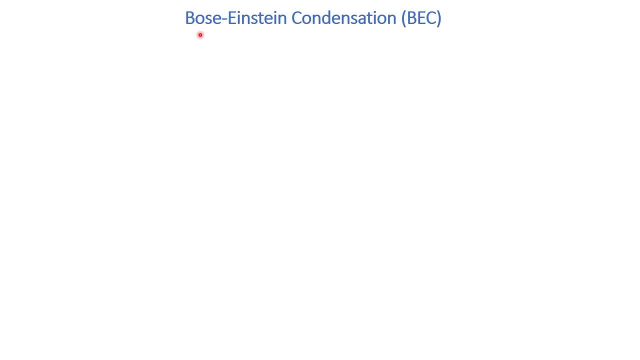 And a state is reached. at a certain lower temperature, all the bosons occupy the ground state of the system, And this gives rise to a new state of matter that is known as the Bose-Einstein Condensate. The idea of Bose-Einstein Condensation arose in 1924, when Bose was working on the group of photons. 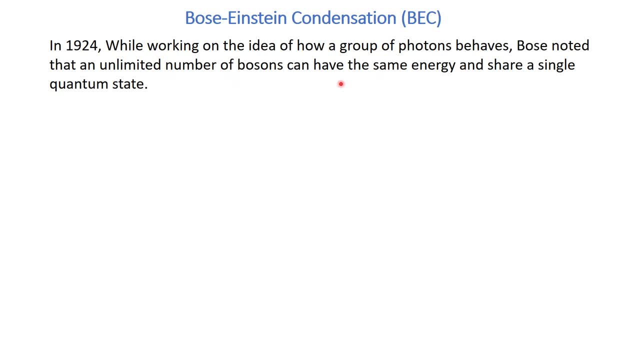 He noted that an unlimited number of bosons can have the same energy and share a single quantum state. Bose sent his work to Einstein and Einstein extended the work of Bose to show that at extremely low temperature the bosonic atom would group into a shared quantum state at the lowest available energy state. 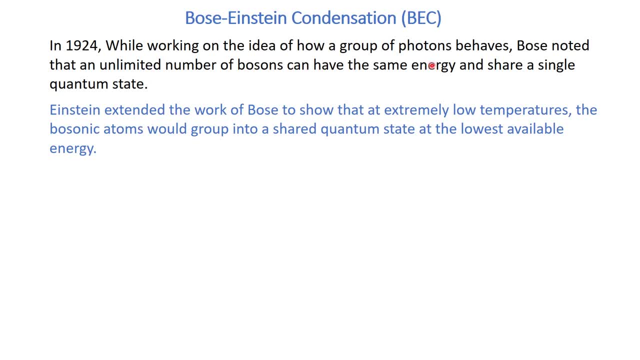 Bose's work was on the photons. However, Einstein extended it to all the bosons. And from the bosonic atom we mean that the atoms which have integral spin, For example the atoms with zero spin- 1,, 2, and 3, they are all bosonic atoms. 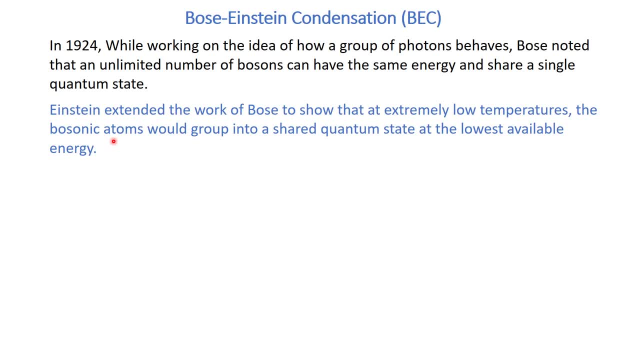 While the permianic atoms are those atoms which have spin equal to 1⁄2, 3⁄2,, 5⁄2, and so on. For example, hydrogen has a spin of 1⁄2, so that is a permianic atom. 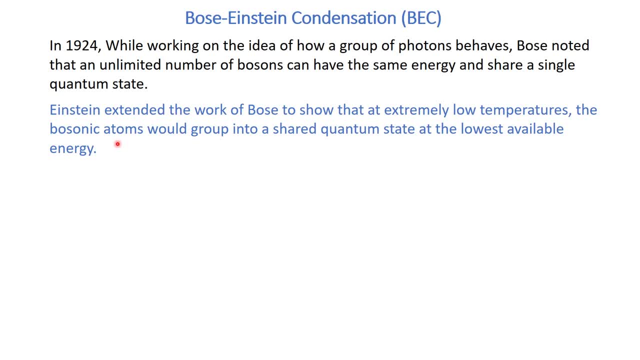 While helium has a spin of 0, so it is a bosonic atom, And this forms a new state of matter which is known as the Bose-Einstein Condensate, And the phenomena itself is known as the Bose-Einstein Condensate. 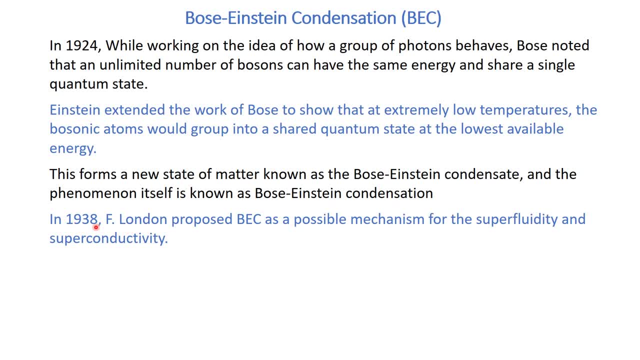 As I explained earlier, In 1938, a scientist known as F London, who proposed that the Bose-Einstein Condensation could be a possible mechanism for explaining the phenomena of superfluidity and superconductivity. In 1995, the Bose-Einstein Condensate was produced in labes by cooling the rubidium atom below 100 degrees. 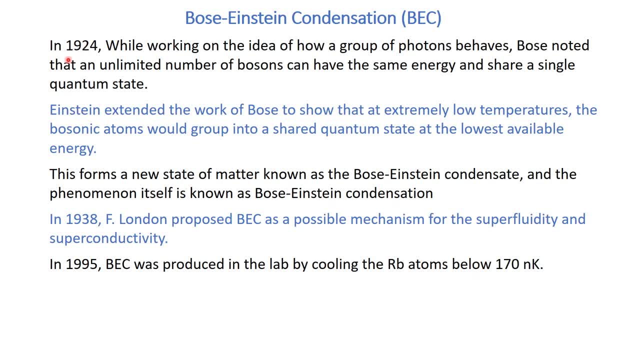 So the idea was floated in 1924.. However, experimentally the Bose-Einstein Condensate was obtained in the labes in 1995.. There were some experiments to know about the properties of the Bose-Einstein Condensate in 1999 and 1998.. 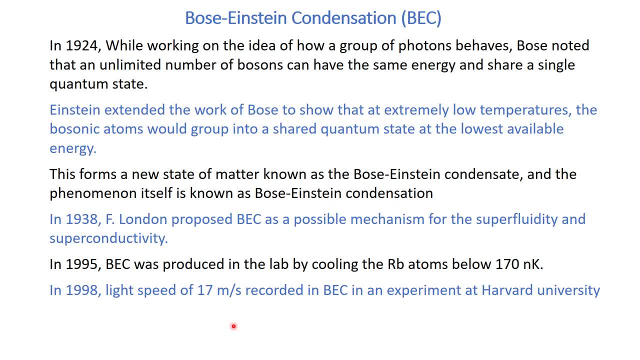 In one such experiment at Harvard University, it was noted that the speed of light is extremely reduced when the Bose-Einstein Condensate is equal to 17 meters per second. So that is extremely low speed for the speed of light in the Bose-Einstein Condensate. 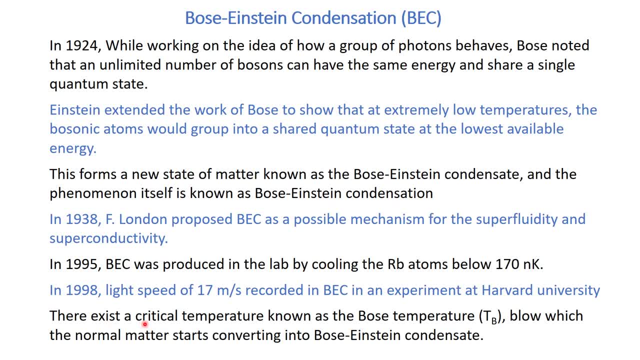 For the Bose-Einstein Condensation there exists a critical temperature that is known as the Bose temperature, represented by Tb, below which the normal matter starts converting into the Bose-Einstein Condensate. So you can call this Bose temperature as the critical temperature. 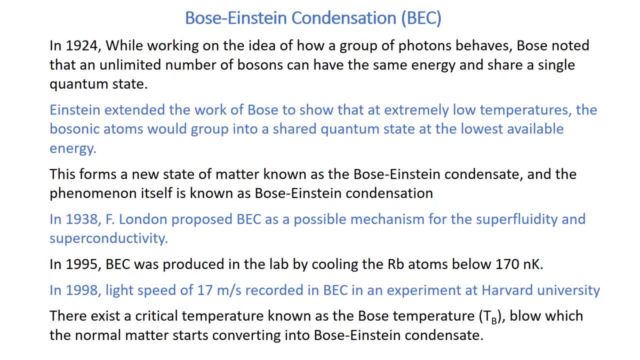 This is from where the phase transition starts: from the normal matter to the Bose-Einstein Condensate. Just like when we go on decreasing the temperature of water so below zero degrees centigrade, the water starts converting into ice. That is the solid state. 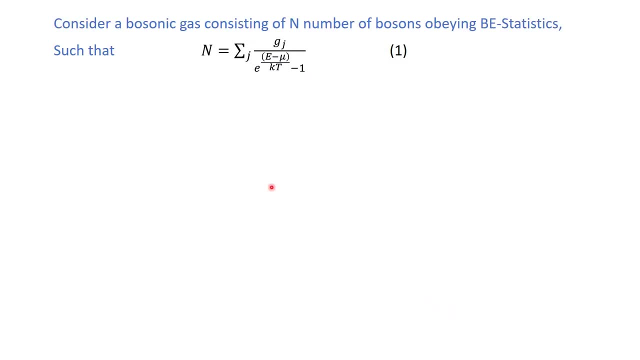 Now we are going to discuss certain properties of the Bose-Einstein Condensate, and for that we have to take help of the Bose-Einstein Statistic. So according to the Bose-Einstein Statistic, the number of bosons and occupying the Bose-Einstein Statistic could be written as this: 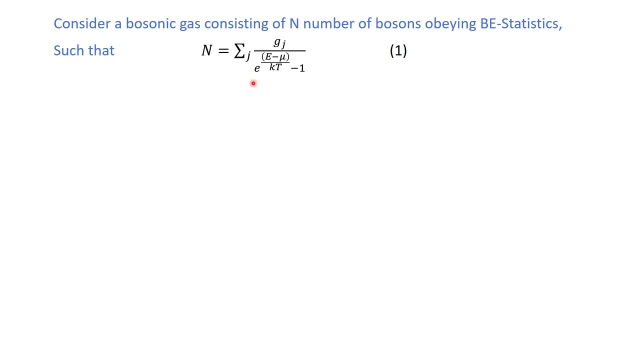 where Gj is the degeneracy, E is the energy of the state and Mu is the chemical potential And K is the Boltzmann constant and T is the absolute temperature In general, the energy of the quantum state. already closed this space. 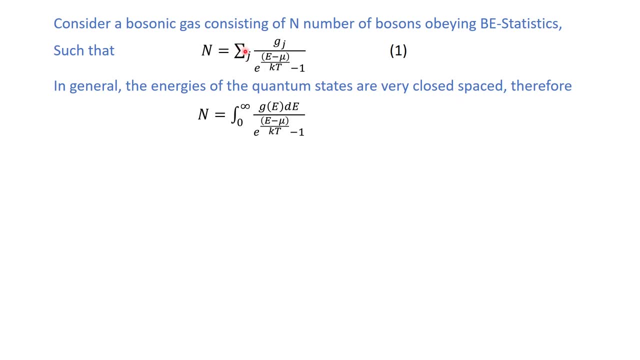 so we have to replace this summation by integration. So equation number one can be written as this: where Gude is the number of energy states between the energy E and De, and we have already calculated Gude while we were discussing the Boltzmann elastic distribution. 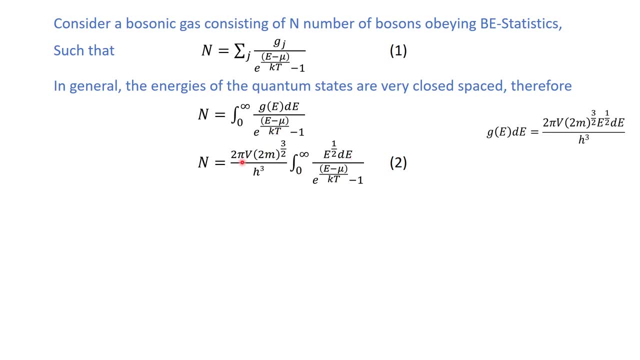 So here you can take all the constants out of this integral and you have to calculate this integration there. Now, this equation number two represents the number of particles in the exact state, because Gude is equal to zero at E is equal to zero. 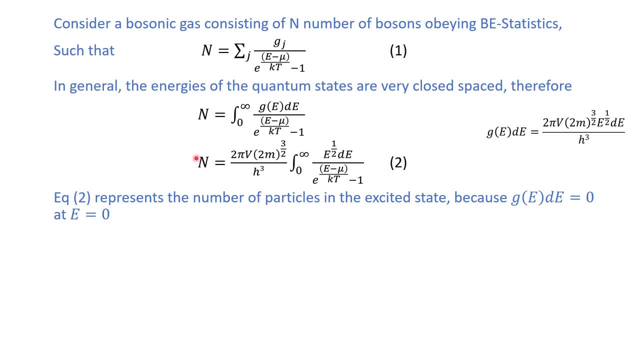 So this integration excludes the number of particles which are in the ground state. So what we can write for the total number of particles is that it is the sum of the number of particles in the ground state plus the number of particles in the exact state. 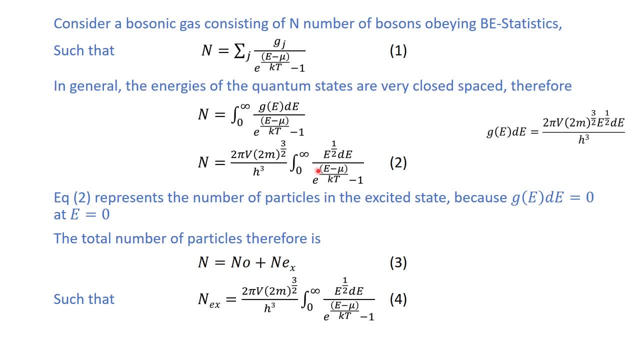 So this equation to actually exclude the number of particles in the ground state, it means that equation two represents the number of particles in the exact state. So we can write equation number two as equation number four, which represents the number of particles in the exact state. 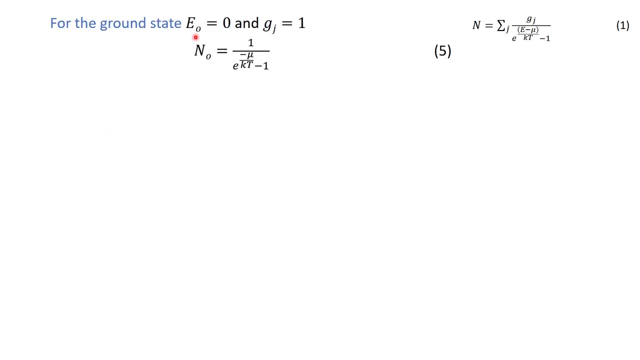 And for the ground state we have E zero. so the energy of the ground state and that is equal to zero, and the ground state, of course, this is the non-digital state, so Gde is equal to zero. So from this equation number one, 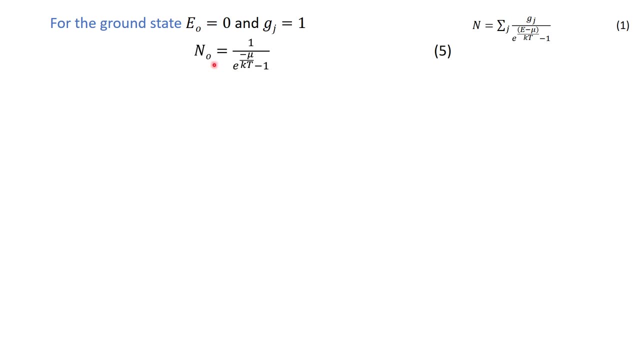 we have N. zero is equal to this, given by equation number five. So equation number five gives the number of particles in the ground state, while equation number four on the previous page gives the number of particles in the exact state Now, at the very low temperature. 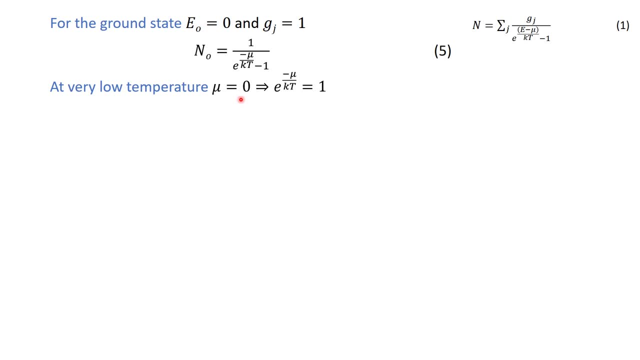 the chemical potential is equal to zero because at very low temperature the energy is quite low. So by adding or removing the particle in a system has no effect on the overall energy of the system. so that is why the chemical potential is equal to zero. 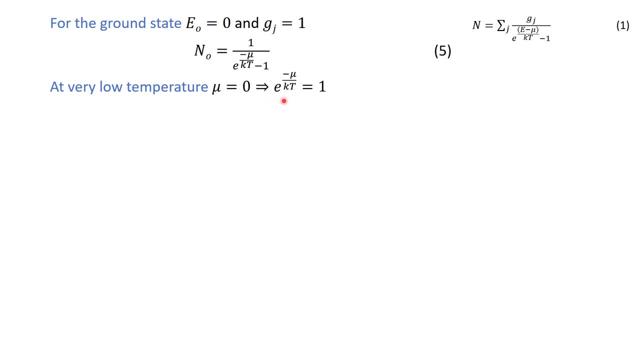 and if the chemical potential is equal to zero, so the exponential is equal to one. And if we put this, exponential is equal to one. so from equation number four we can have the expression for the exact rate number of particles given by equation number six. 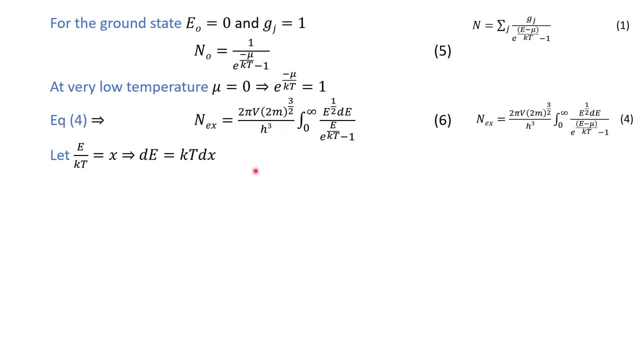 Now we have to solve this integral, and for that we put e to the power. of kt is equal to x, such that d is equal to kt dx. So from equation number six we have this. now we are rearranging. 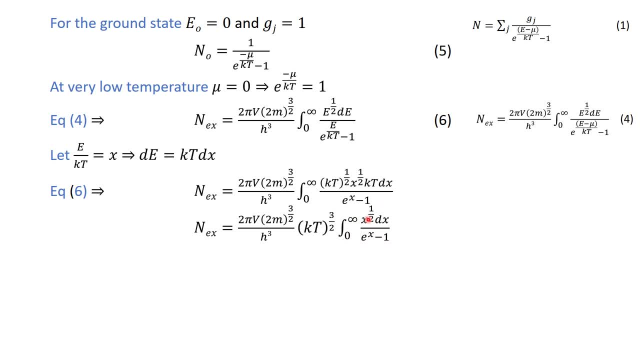 we have this integral, so now we have to solve this integral. If you remember, we have already encountered this integral, such type of integral, when we were discussing the Debye theory of specific heat, and this is equal to gamma three zeta. 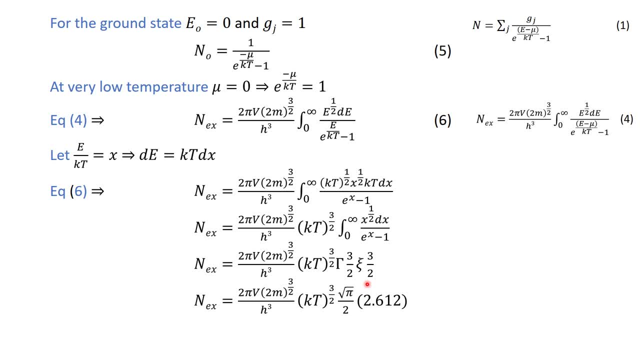 gamma three by two is zeta three by two, and the value of gamma three by two is five under root. two by two and zeta three by two is equal to two point six, one, two. By rearranging this we can write the number of excited bosons. 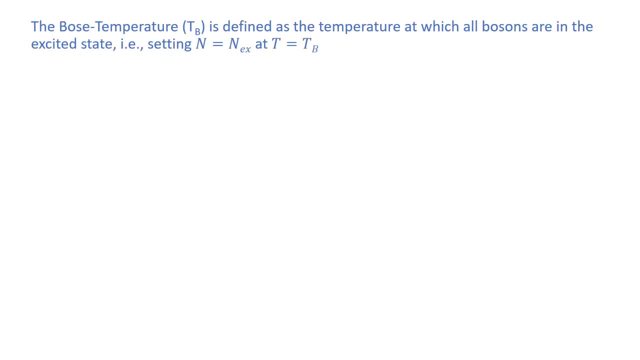 in terms of equation number seven- Now we have the Bose temperature- is the temperature at which all the bosons are in the excited state. This is the critical temperature above which the material exists in the normal state and below which the material starts converting. 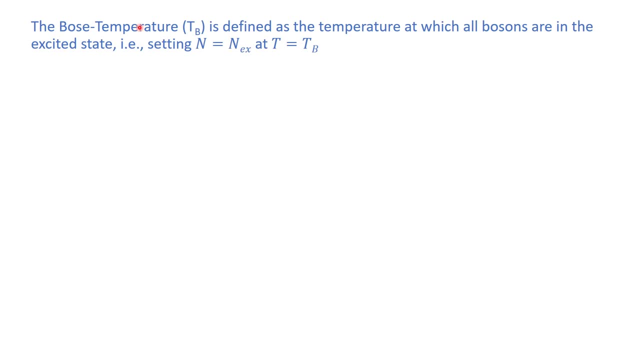 into the boson style condensate. So if we are at the Bose temperature, so the total number of particles are in the excited state. So here in the previous slide you had, n e, x is equal to this by equation number seven. 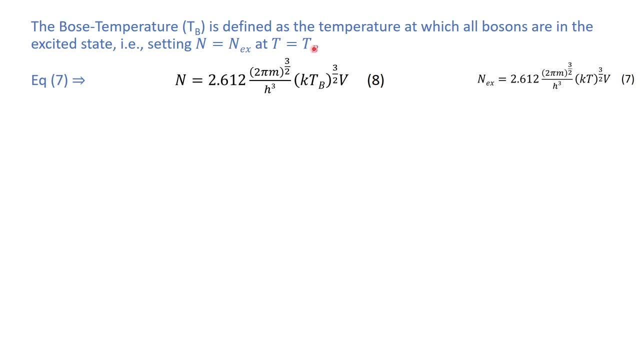 And we have to write the total number of particles of any general temperature, T. But when we put T is equal to T, d. so you can write: n e, x, which is the number of the excited number of bosons, is equal to the total number of particles. 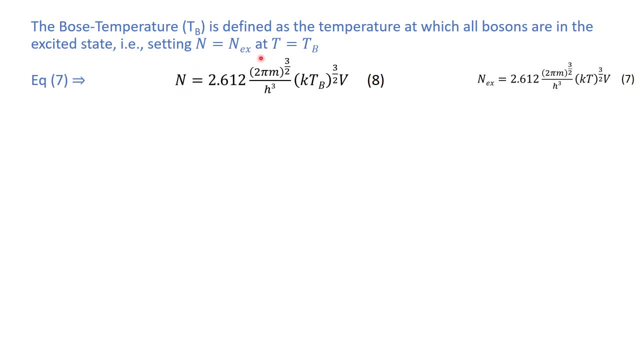 So from equation number seven, when we do this substitution, we have the total number of particles given by equation number eight. Now from this equation number eight that we can calculate the value of Bose temperature. so to rearrange this equation. so you have. 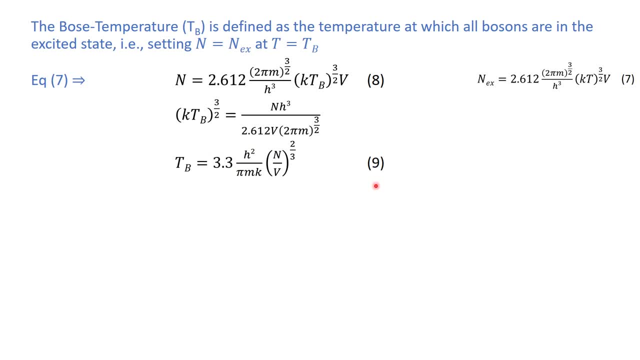 the value of the Bose temperature given by this number. and you see that value of the Bose temperature depends upon the number of particle for unit volume. you know that every metal is different number of particle for unit volume. that is why every metal will have different value of the Bose temperature. now from equation number seven and eight, the ratio. 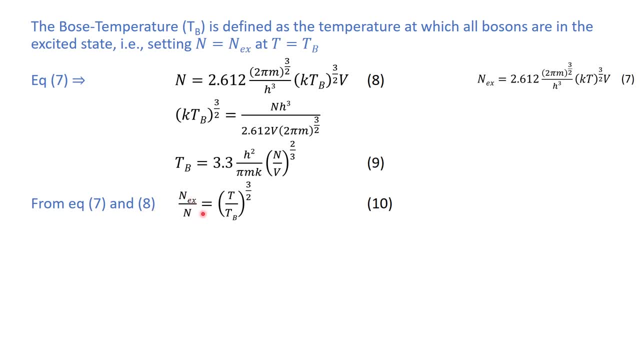 of the exact number of boson to the total number of boson is given by equation number ten, which depends upon the temperature. similarly, you can write this: n e- x equal to n minus n, because we know that total number of particles is equal to the number of particles in the 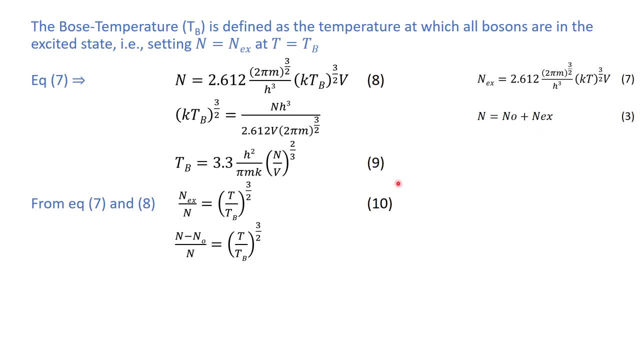 ground state plus the number of particles in the excited state. so the number of particles in the excited state will be equal to the total number of particles minus the number of particles in the ground state. if you rearrange it so you can write the ratio of the number, 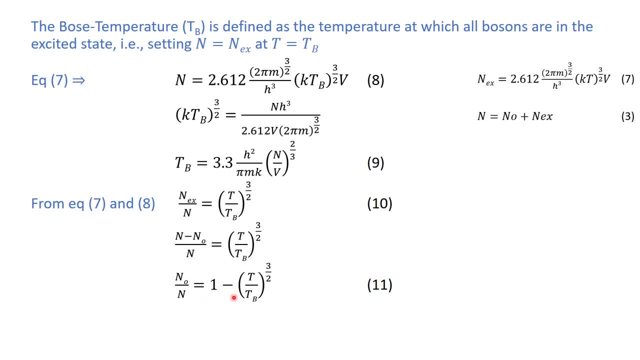 of particles in the ground state towards the total number of bosons given by equation number eleven. so when we are writing the ratio of the number of particles in the ground state, then we are at the Bose temperature. so from equation number ten, n, e, x equal to n, that is, 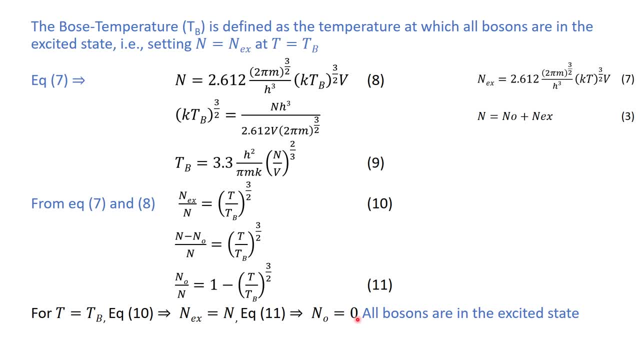 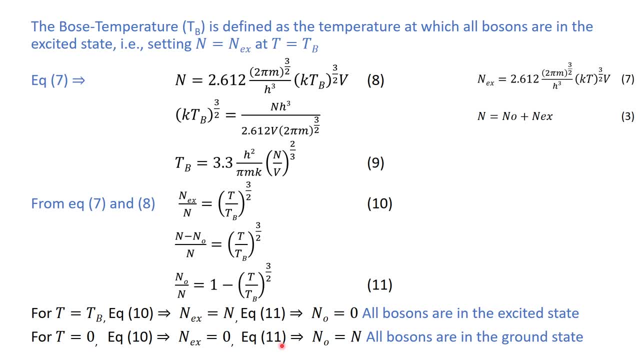 0 and the equation number ten shows that the ground state particle will be equal to n. that is all the bosons will be in the ground state. so the transition from the normal method towards the both Einstein, Kornstein start at temperature, below both temperature and at absolute zero. 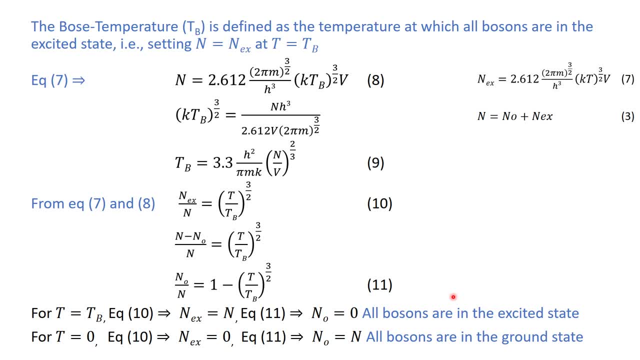 the material is completely converted and the boson stand condensate. however, at the temperature between the absolute zero and the boost temperature, there is a mixture of the boson stand condensate and normal matter. this you can see from this plot. so the, the dash line represent the number of particle in the excited state and 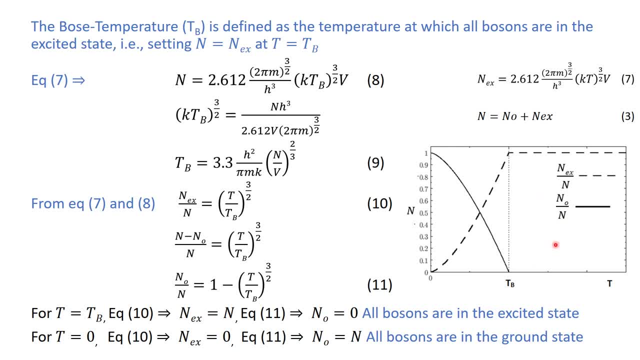 the solid line represent the number of particle in the ground state. so when you are at that temperature- above the boost temperature, so this ratio is equal to one- mean that all the particle are in the excited state. however, when you go below the boost temperature, so the ratio of the excited. 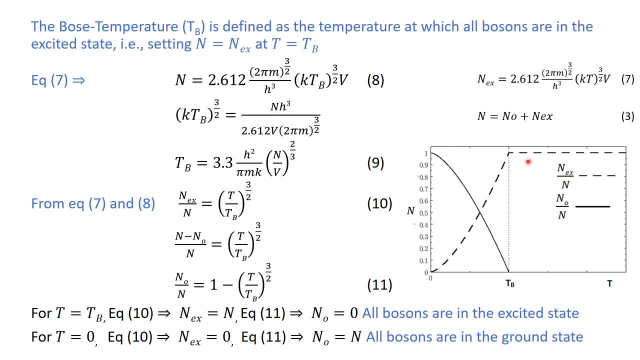 number of particles toward a total number of particle go on decreasing. it means that the excited particle go on decreasing and it go on decreasing until it goes to zero, at the absolute zero. at the same time when the excited particle go on decreasing, the number of particle in the ground state go on increasing. 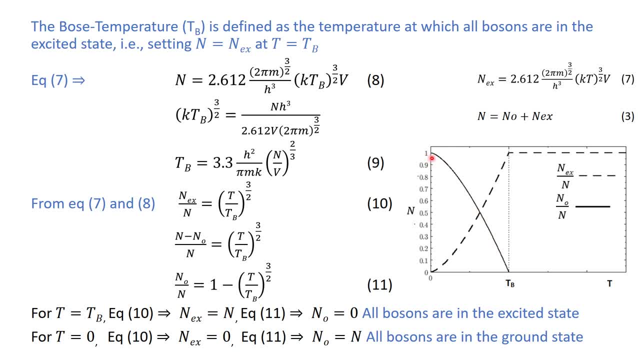 and at absolute zero. it this ratio goes to one, it means that now the total number of particles are in the ground state. so here this is a mixed state, where we have some particle in the ground state and some particle are in the excited state. however, here, in this case, there is no particle in the 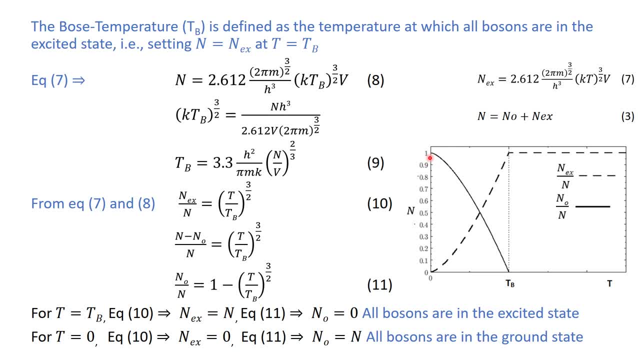 excited state, while all the particle are in the ground state. so this is the pure Bose-Einstein condensate. this is the mixed state and this is the pure normal matter state. so this was all about the Bose-Einstein condensation. we have covered the main part of your syllabus. however, it still 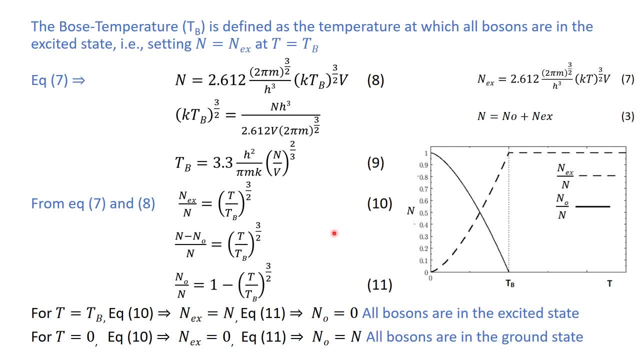 have some problems which we can discuss later on. okay, thank you, love you.